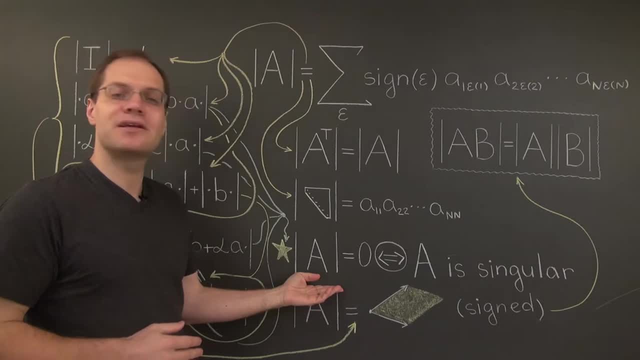 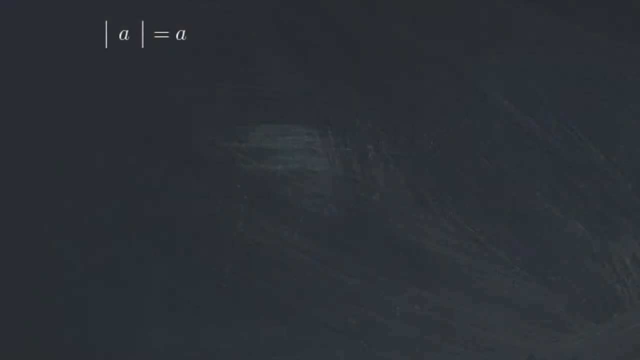 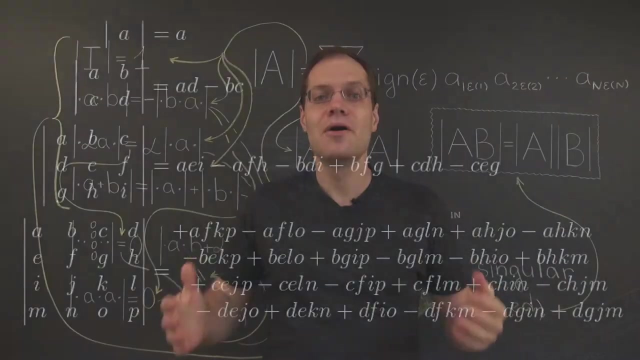 determinants of small matrices based on this property. right here, And here are the expressions we came up with, Here is the one by one, the two by two, the three by three and the four by four. determinants Now based on these. 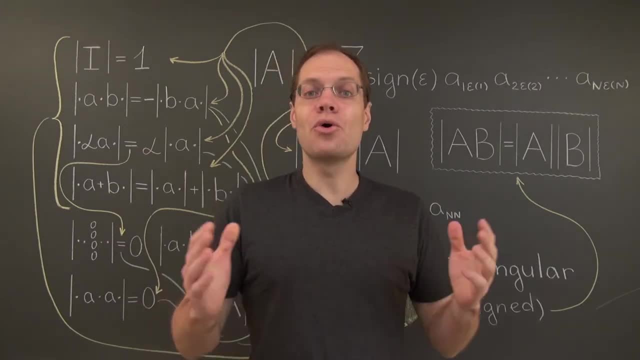 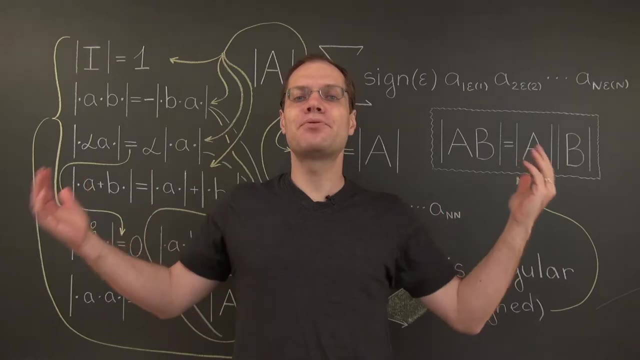 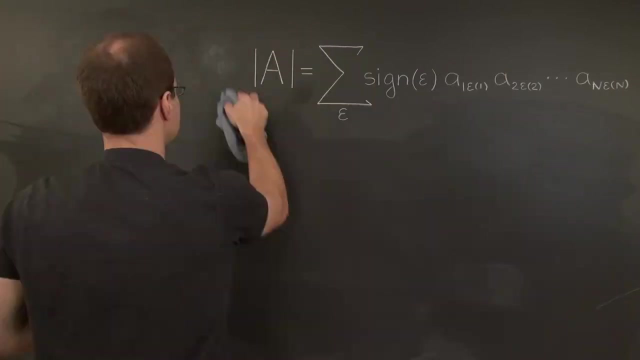 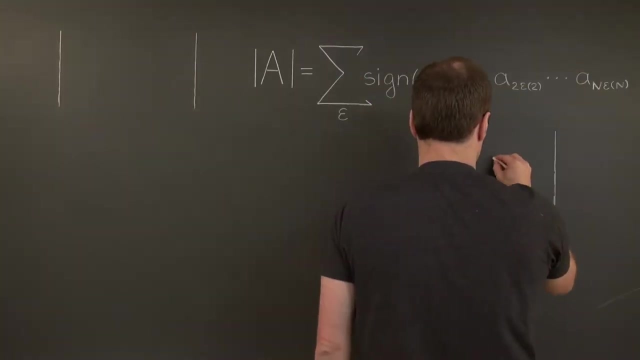 expressions. we're going to postulate, or guess if you will, this algebraic definition, And then we'll go from this definition to the properties of the determinant. So let's get started. Subtitles by the Amaraorg community. Now, in order to make the pattern that's emerging from the available expressions. 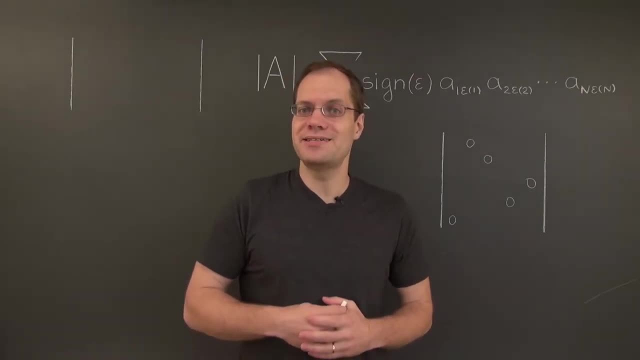 clearer. let's switch from denoting the entries of the matrix by different letters to denoting them by the same letter a, and letting a pair of subscripts indicate the entries position in the matrix. By convention, the first subscript indicates the row and the entry position. 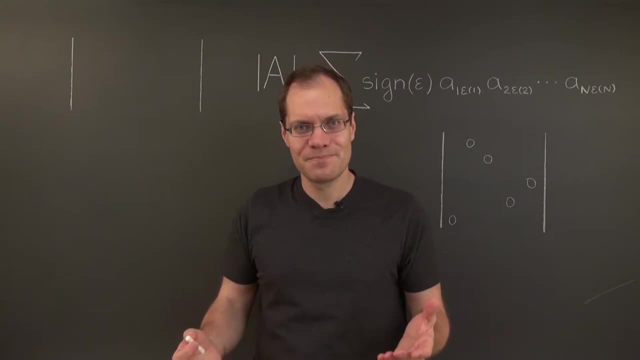 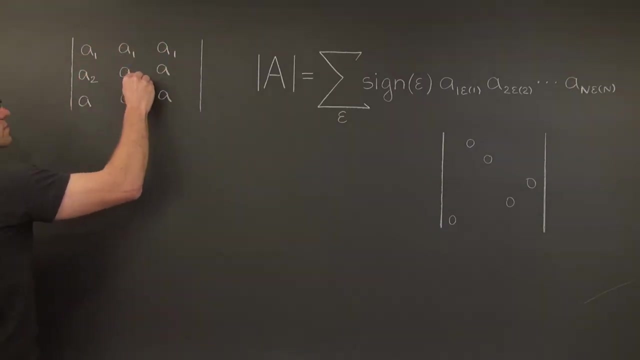 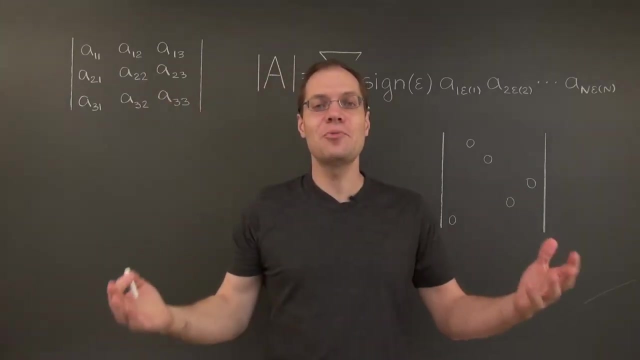 Subtitles by the Amaraorg community. And the second subscript indicates the column. So a three by three matrix becomes this, And pay attention to the order in which I'm writing the subscripts. Subtitles by the Amaraorg community. I hope it was helpful to watch that matrix unfold And I also think it'll be. 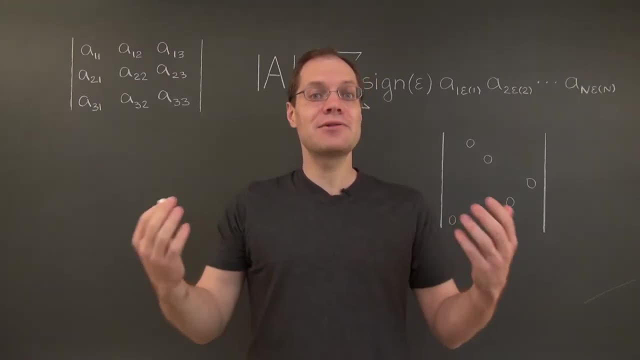 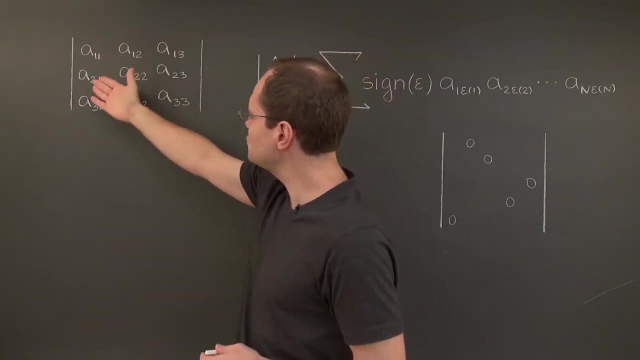 helpful to hear the information that's being given to us in order to be able to learn the entries of the matrix read out loud. So let's go row by row. We have a one one, a one two, a one three, a two, one, a two, two, a two three and a three one. 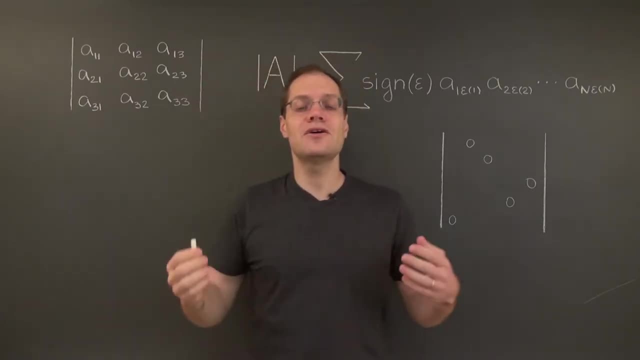 a three, two, a three, three. So when you hear of the entry a two, three, you immediately know that it's the entry in row two and column three. Or in a larger matrix, if you hear a seven twelve, you know that it's the entry in the seventh row. 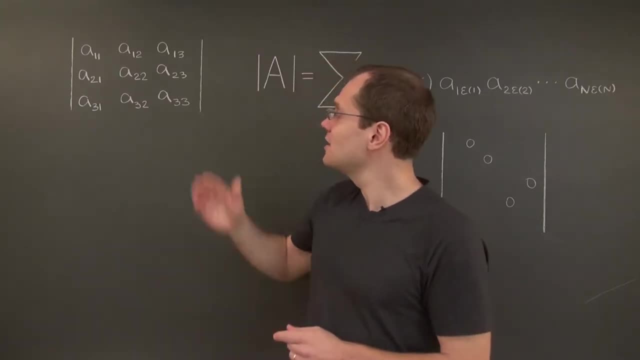 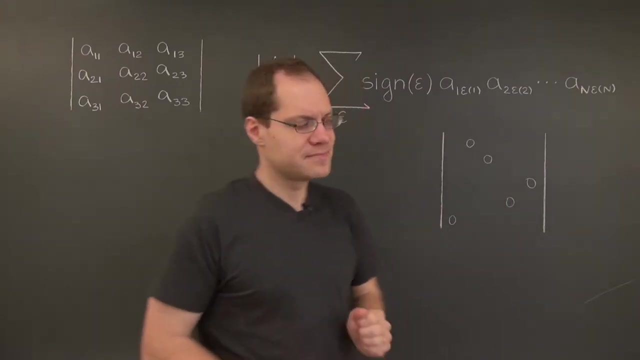 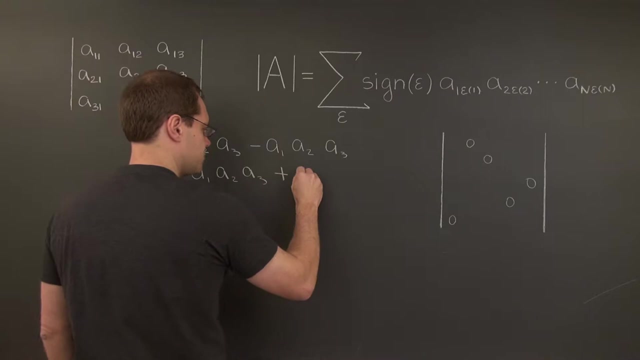 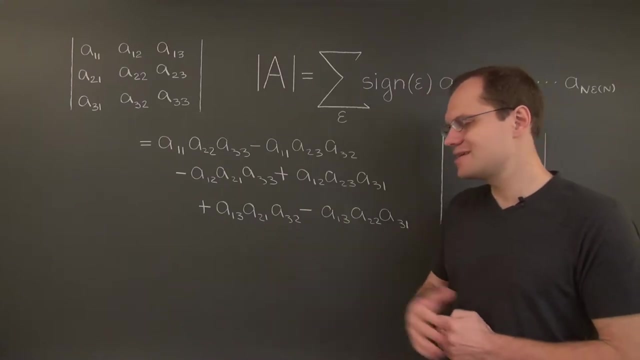 the 12th column. Now let me write down the determinant of this matrix using these new symbols, And once again pay attention to the order in which I write the subscript, And I believe the pattern summarized by this definition will begin to emerge. Okay, I will leave it up to you to make sure that this expression is correct. I 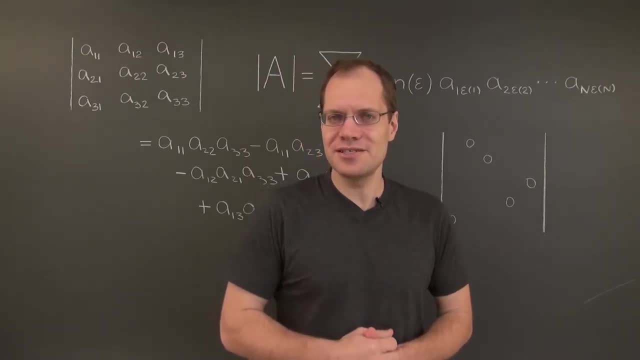 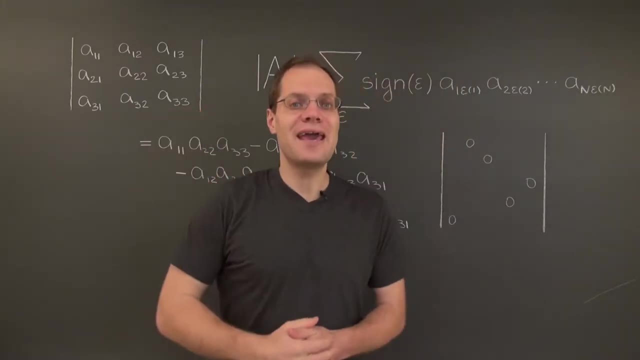 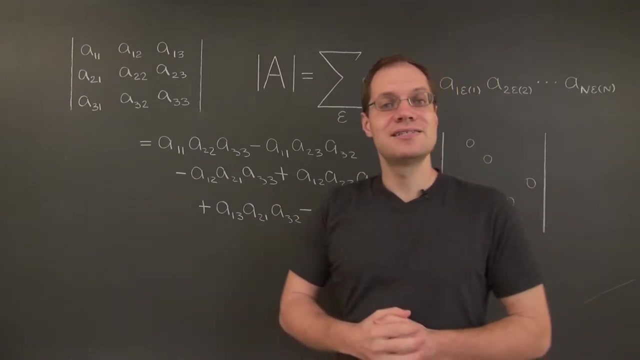 recommend thinking back to the Russian way of calculating 3x3 determinants and verifying that these terms correspond to the correct six patterns. Okay, now it's time to take a step back and to summarize what we're seeing. We have six terms each. 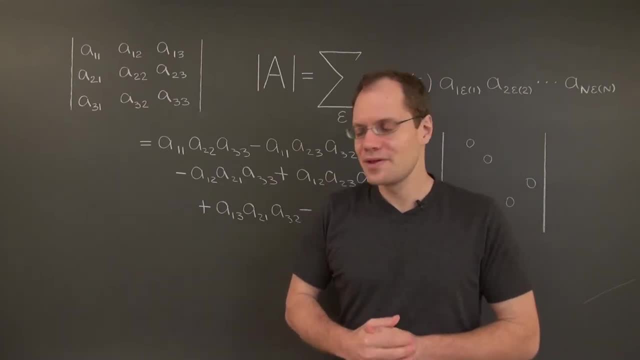 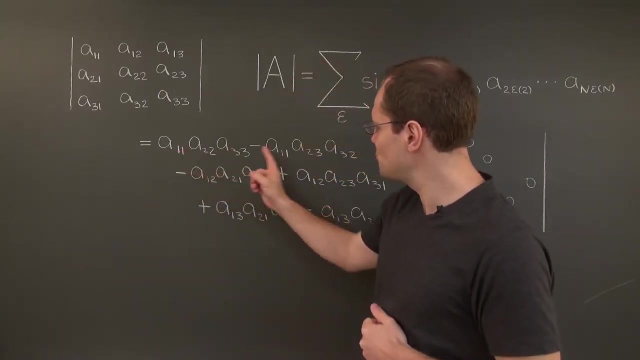 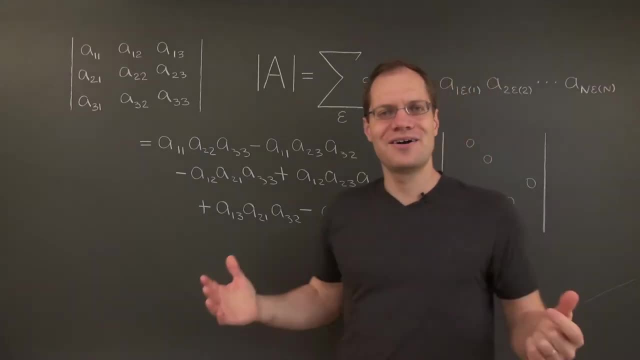 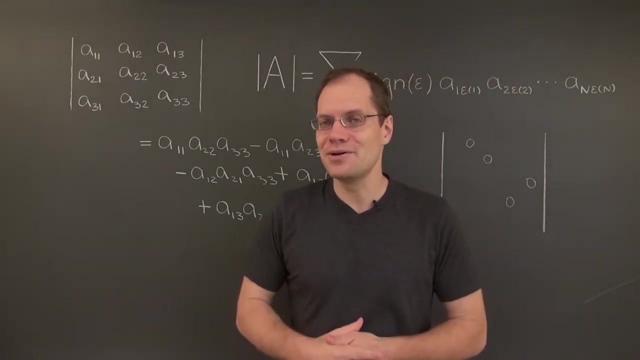 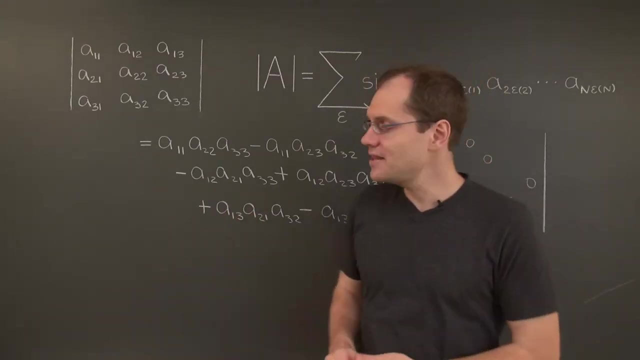 3, 1, 2, 3, 1, 2.. All right, what about the columns? Well, the columns are totally different. The columns are completely scrambled, except in the first term. The columns correspond to permutations, And that's why we have six terms, because there's six possible. 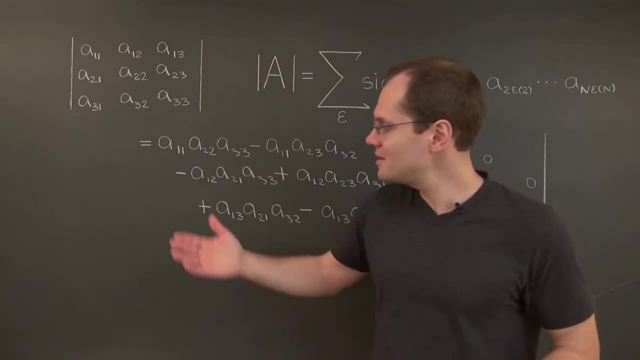 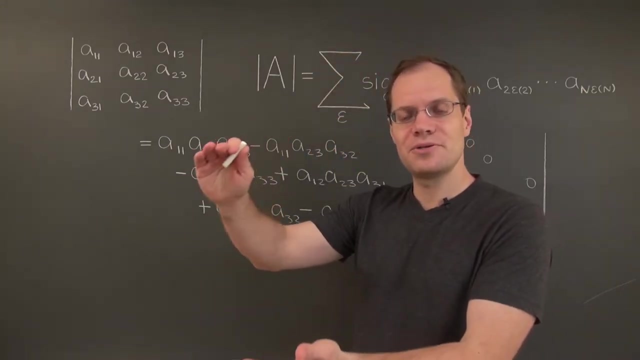 permutations of numbers 1,, 2, and 3.. Let me write each of the permutations down, And I think you should do the same. You should pause the video, write down all the possible permutations of numbers one, two and three, find a system for doing that and then come back and check with us. 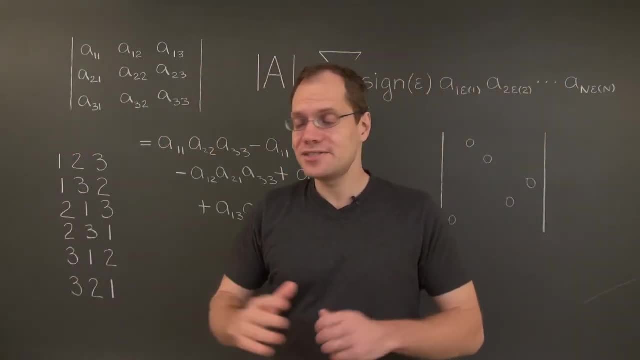 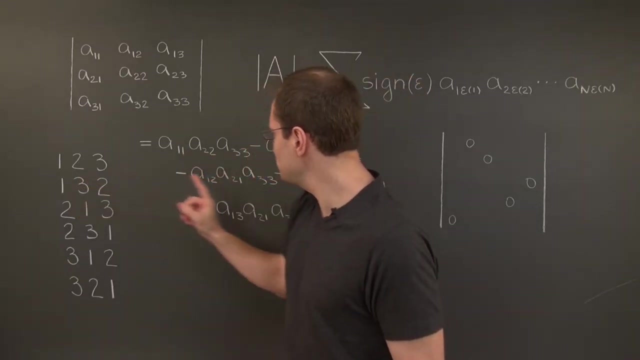 all right, there you have it, and now you see how there is one term corresponding to each of the permutations. you just look at the columns. we have one, two, three. so in the first term the columns go one, two, three, one, three, two, one, three, two, two, one, three, two, one, three, and so forth. 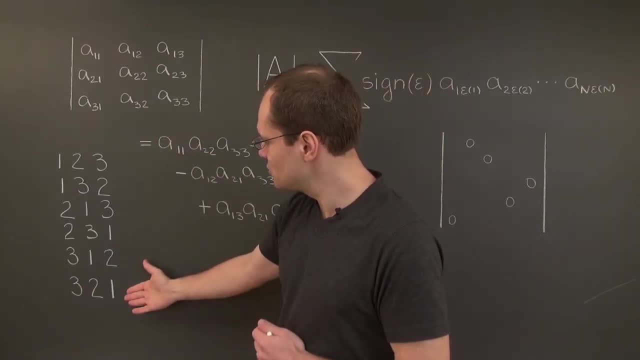 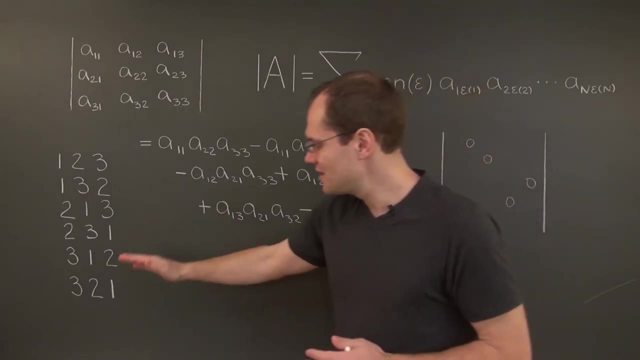 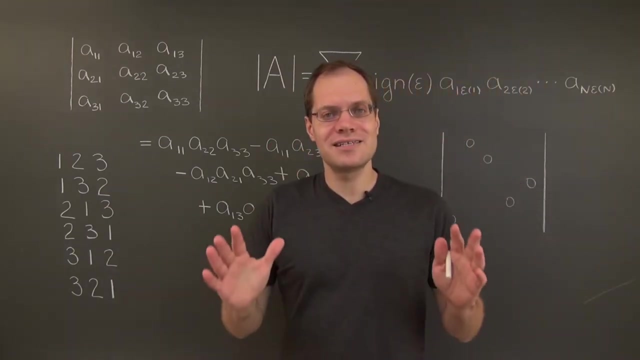 and you can see how i was very systematic about this approach. first i did the terms, with ones in the first place, then with twos, then with threes and in higher dimensions it would be a much longer list. okay, now we understand the terms. the only thing that's left is the sign. 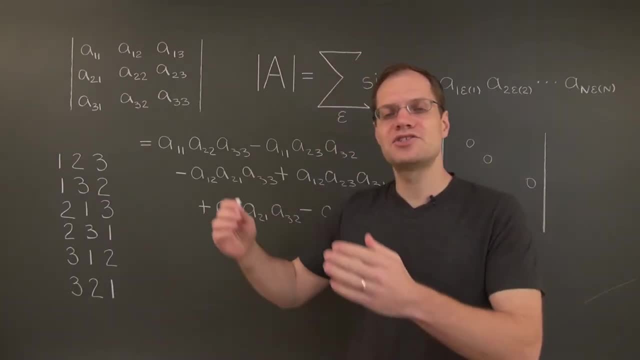 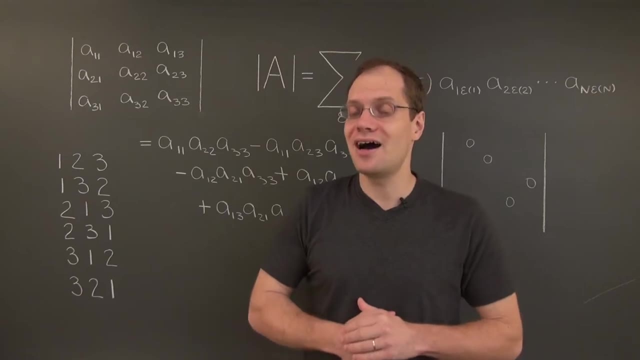 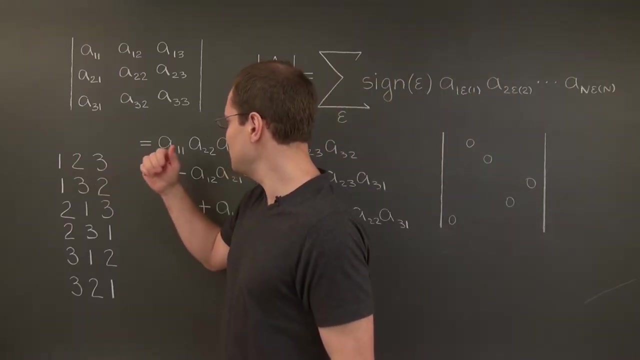 and the sign is very simple: it corresponds to the parity of the permutation. if the permutation is even, it's a plus, if the permutation is odd, it's a minus. so let's see what we have for these permutations: one, two, three is an even permutation, so there is a plus. one, three, two is a single. 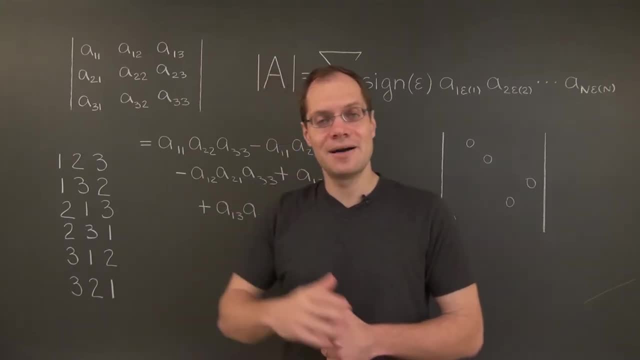 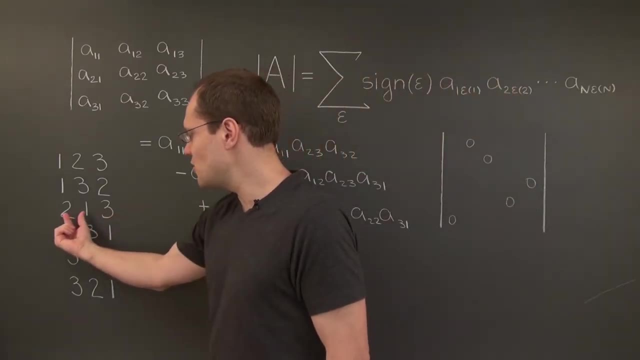 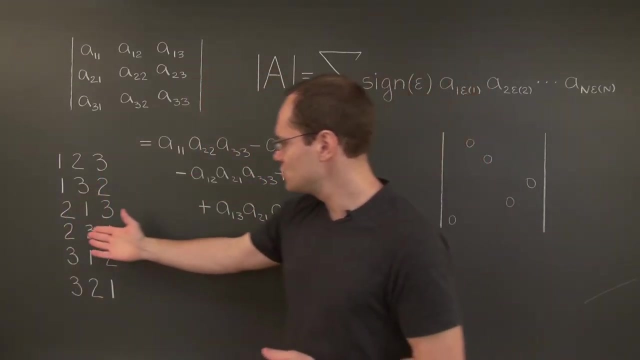 switch away from one, two, three. an odd number of switches. one switch, so it's an odd permutation, so there's a minus two. one, three is also a single switch from one, two, three. it's an odd permutation, so it's a minus two, three. one is two switches away from one, two, three. first we have to swap. 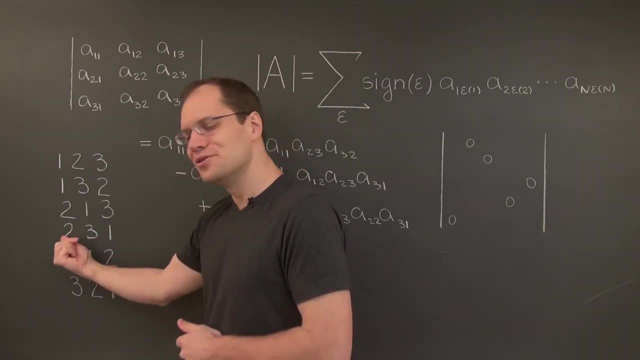 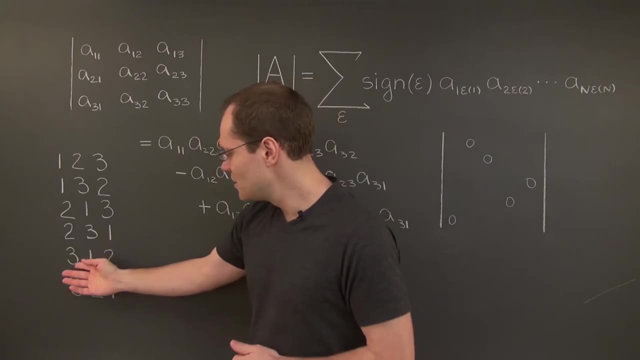 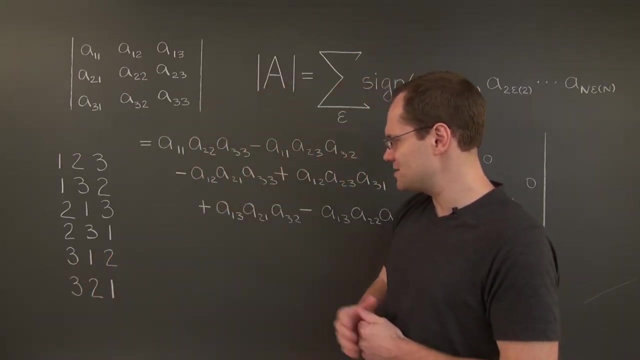 one and three, and then one and two, and we'll have one, two, three, two switches and therefore it's a plus. let's complete the two remaining ones. we have three, one, two- it's one to put the one here and then the other switch to put two and three in their places. so it's a plus, and 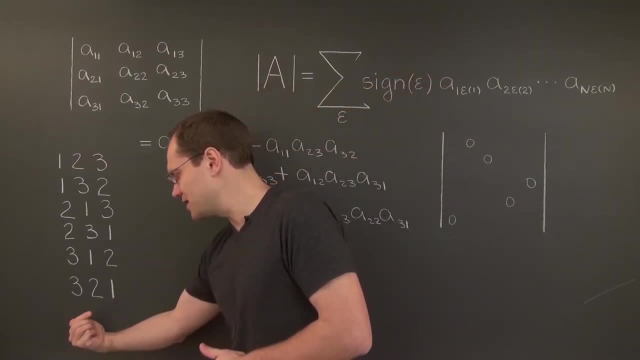 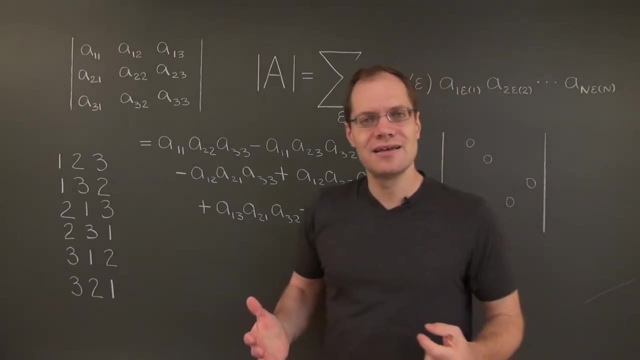 Finally, this one is a single switch swap. one and three away from one, two, three. So it's an odd permutation and there is a minus. so the sign is determined by the parity of the permutation. So it's a plus if it's an even permutation and minus if it's an odd permutation. 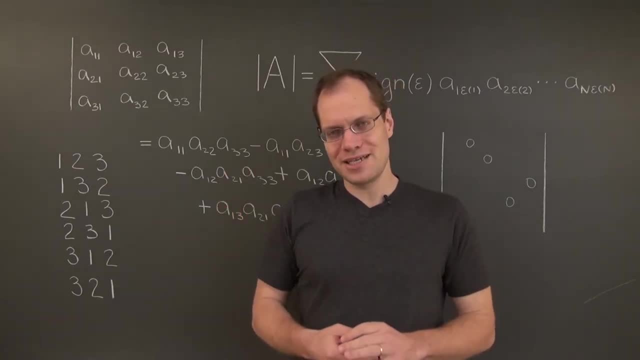 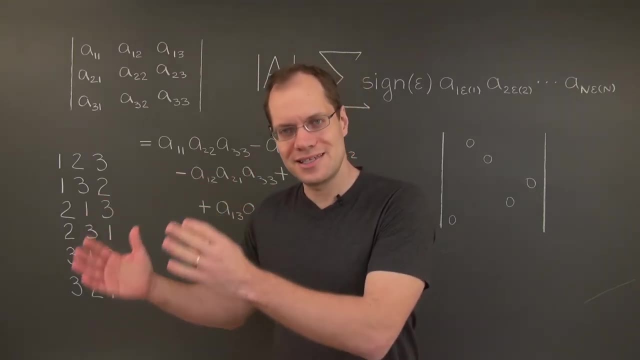 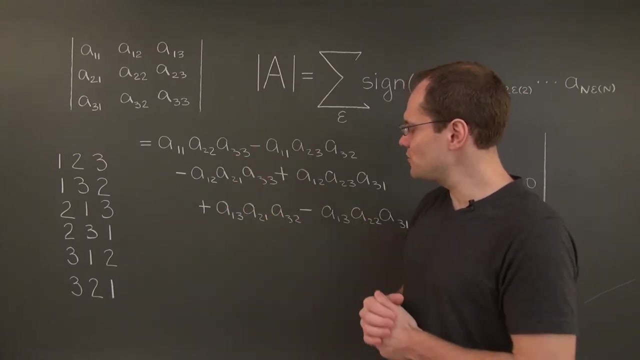 That's actually called the sign of the permutation or the signature of the permutation. You can say that the sign of the permutation is one when it's an even permutation and minus one when it's an odd Permutation. and this completes the statement of the formula for three by three matrices. 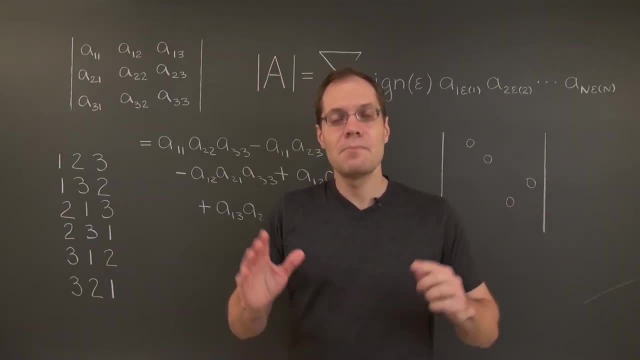 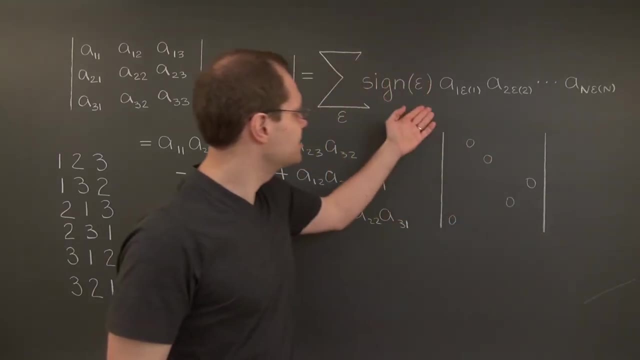 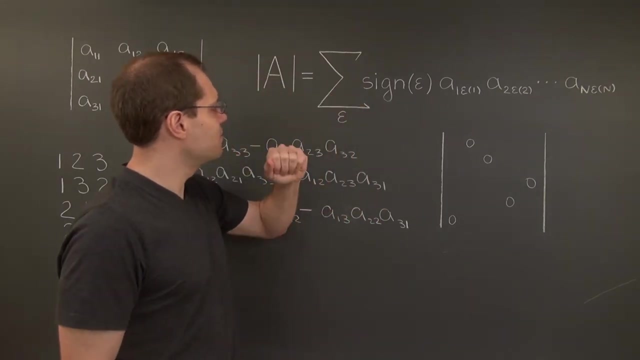 I will now repeat the exact same thing, but I will use words that apply to matrices of arbitrary size and That will pretty much Spell out this formula. Let's see: in the case of an n by n matrix, We'll have a sum of n factorial terms, one for each permutation, and epsilon denotes the permutation. 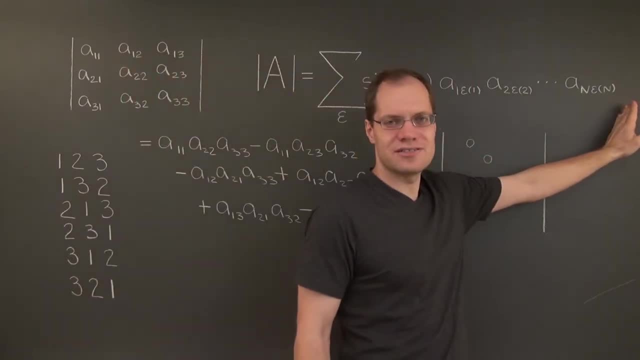 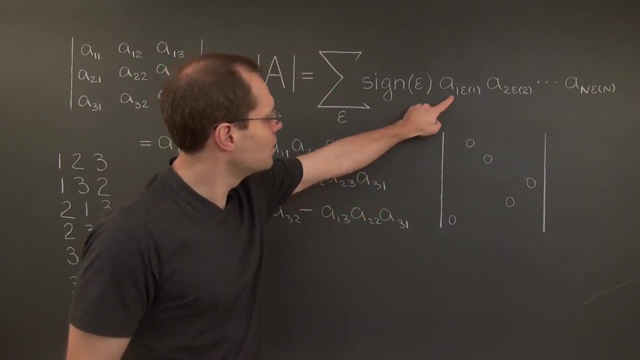 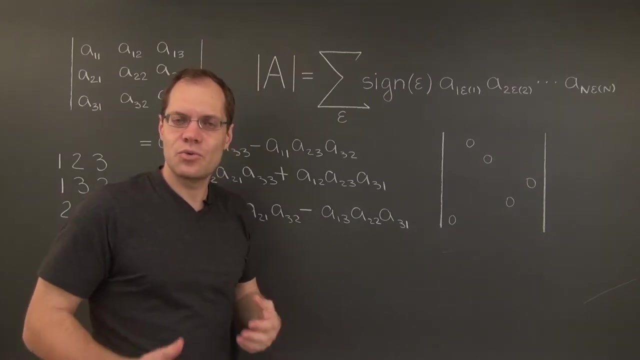 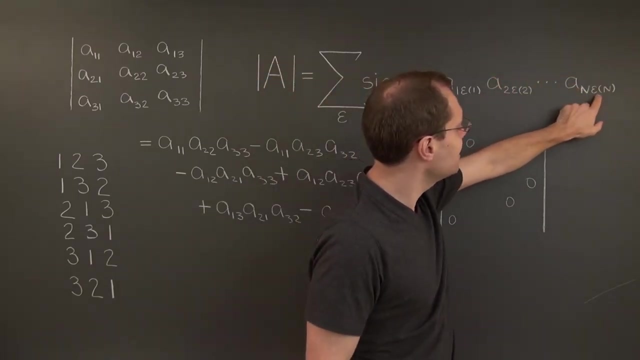 Each term will be a product of n entries, one from each row and one from each column. The rows will come in order. They'll go one, two, three and So forth, all the way to end. the columns will correspond to permutations. That's why I have epsilon of 1, epsilon of 2 and so forth. epsilon of n because epsilon of 1. 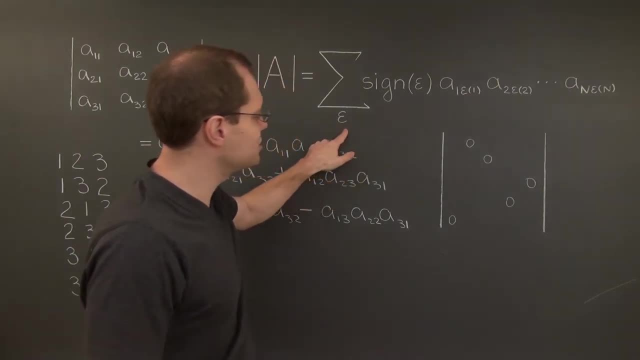 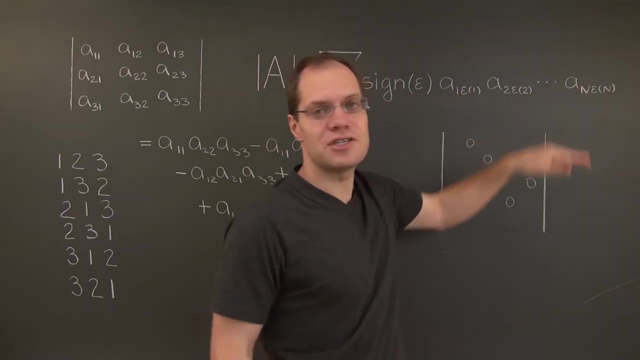 determines the first number in the permutation epsilon, This is the second number And this is the nth number. so you can see how. this is a straightforward generalization of what we saw in the case of three by three matrices. and finally, the last element to be found is our. 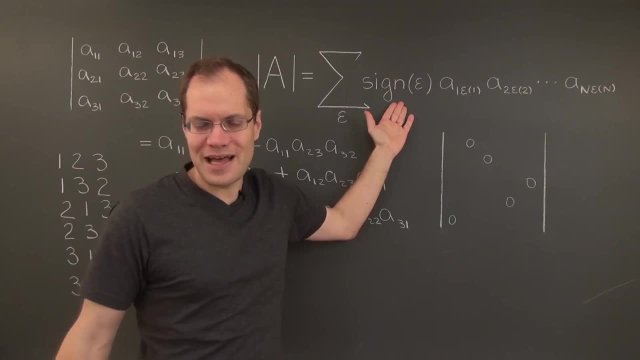 is the sign, And it's the sign of the permutation. I've already said it several times. Let me say it one more time: It's a plus if it's an even permutation, and it's a minus if it's an odd permutation. So there you go. That's the general definition. Let me show you on. 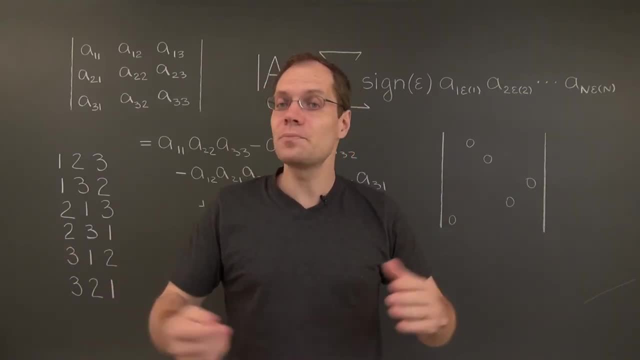 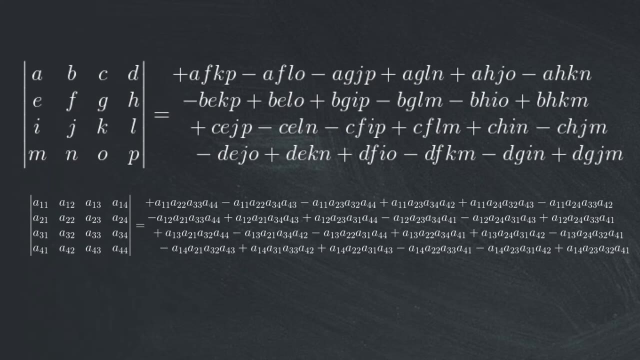 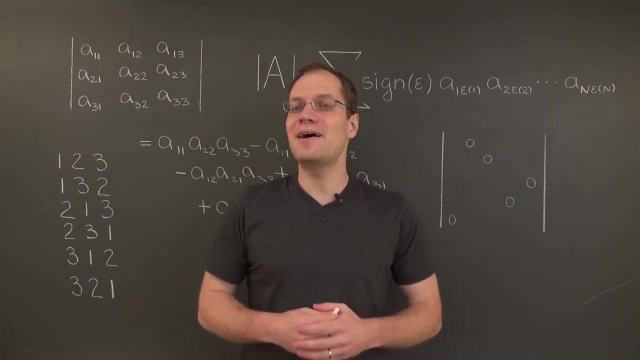 the screen what this definition results in for 4x4 matrices And you can make sure for yourself that each of the terms conforms to this pattern and comes with the right sign. And finally, a short illustration for 5x5 determinants. We're going to look at a single. 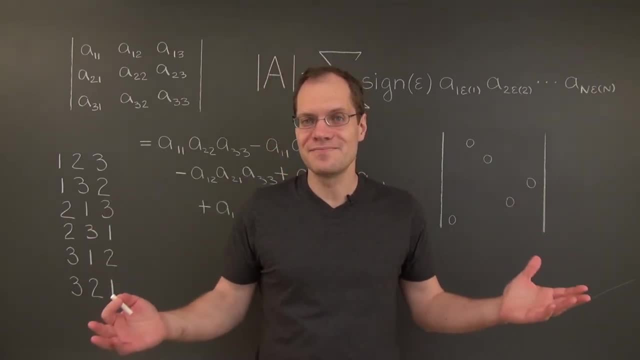 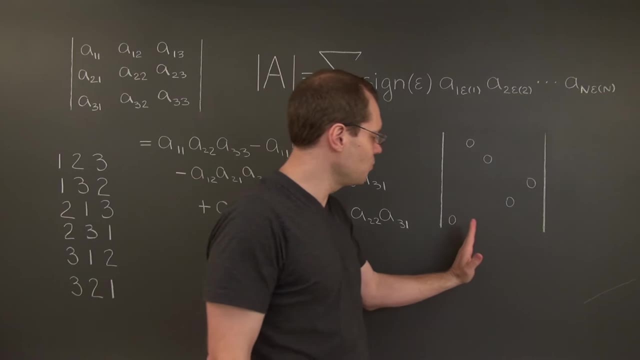 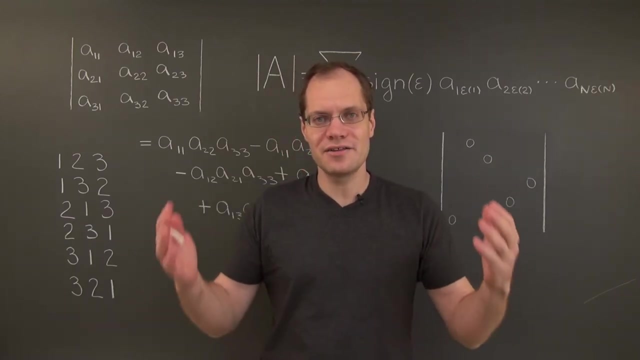 term that I marked on the board out of 120.. And you can see how I selected the entries. So there's exactly one in each row and exactly one in each column, And there are 119 other ways of doing this Corresponding to the other 119 terms in the sum. This one corresponds to the permutation. 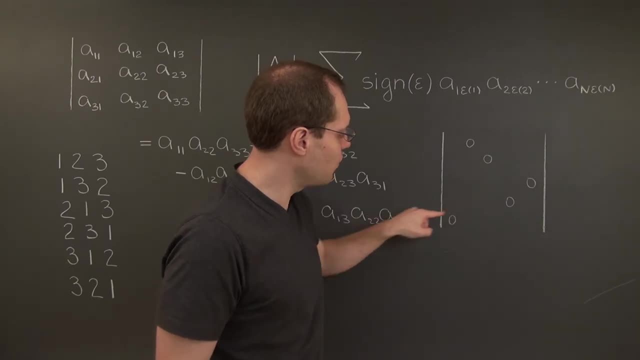 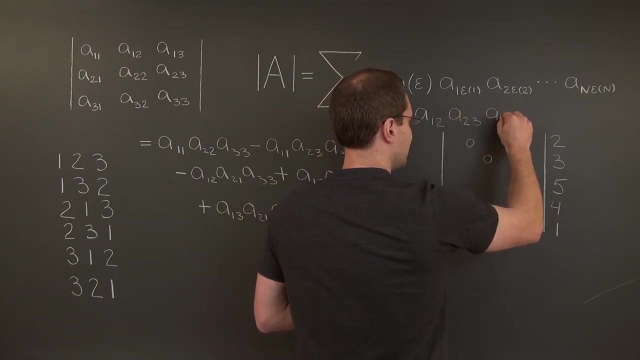 2,, 3,, 5,, 4,, 1.. And so it's the term a 1,, 2,, a 2, 3,, a 3,, 5,, a 4,, 5,, 6,, 7,, 8,, 9,, 10,.